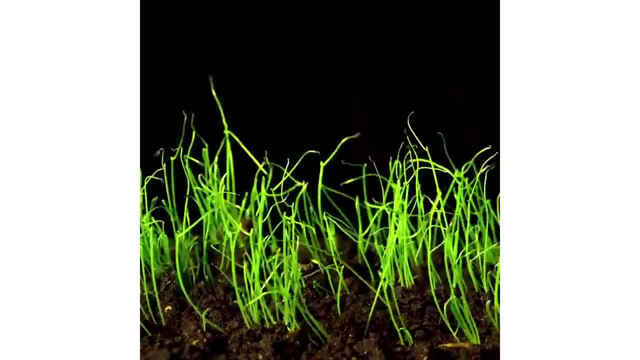 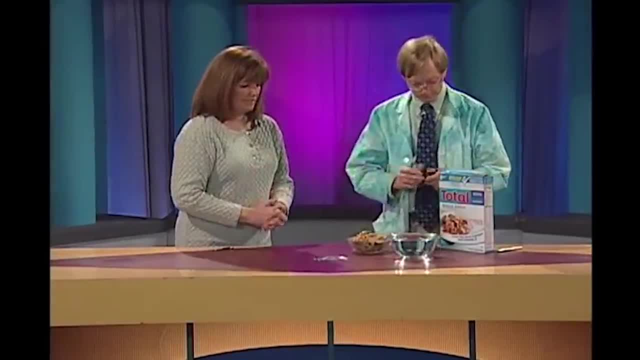 And for onions plant in the center of soil and water regularly. Pretty basic stuff but really awesome results. 22. Magnetic Cereal. If you didn't know already, cereal is a great source of iron and some cereals with high. amounts of iron include honey, bunches of oats, ketlogs, Cheerios and even Chex. All are great for this experiment. It's a 50% chance that you'll be able to get the right amount of iron. It's a 50-50 chance this will work for you, but if you place a magnet over a piece of 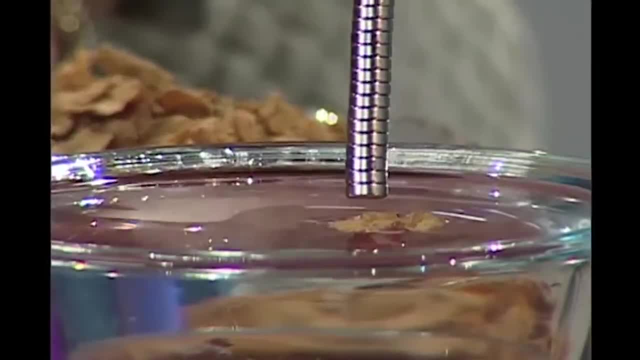 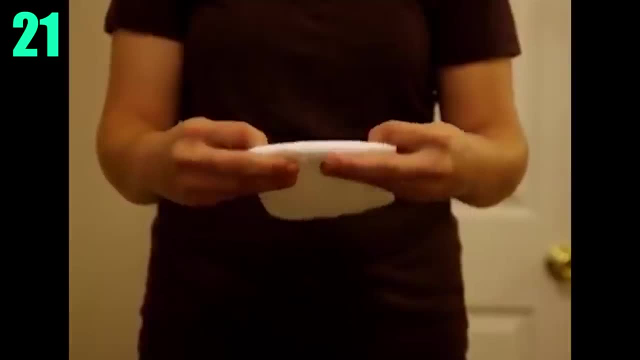 cereal floating in the water. you can manipulate the cereal to follow the magnet, because iron is metal, Just in case you didn't know. 21. Green Money- It's not what you think. You're literally just turning your copper-enriched pennies. 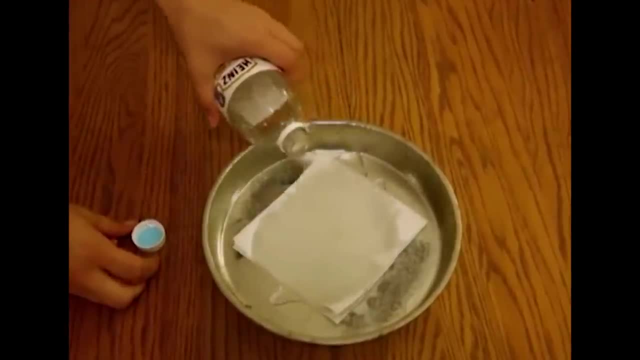 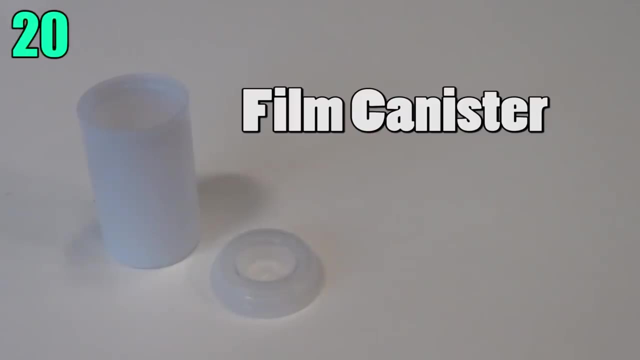 green. Simply dampen the paper towel in vinegar and leave your pennies over it, And over time they'll turn green because it causes the copper to slowly dissolve. 20. Film Canister Rockets. Well, it's not exactly a rocket. 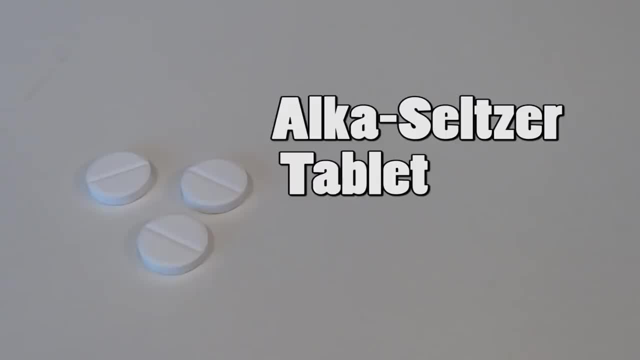 Okay, so all you need is a film canister to fill halfway with water and drop an Alka-Seltzer tablet in the canister, seal it up and, soon enough, the Alka-Seltzer recalls an extreme high pressure buildup and then… it explodes. 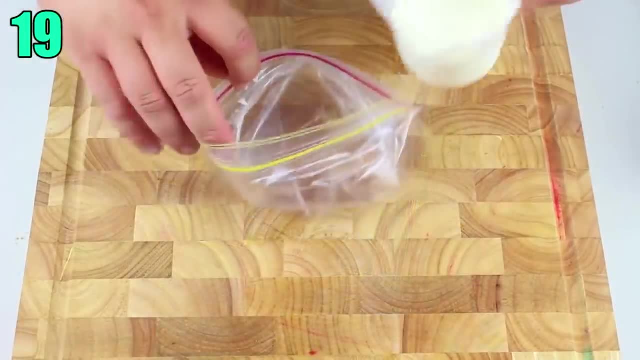 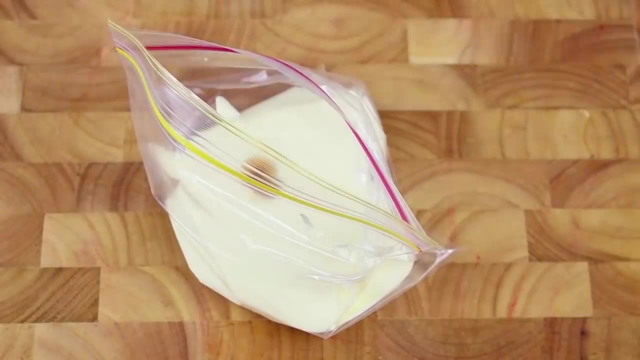 19. Ice Cream in a Bag. There are various methods to doing this experiment, but here's our delicious, awesome version. First, fill a small Ziploc bag with 1 cup cream, 1 teaspoon vanilla extract- for flavor, of course- and 2 tablespoons icing sugar or powdered sugar. both would work, either or In 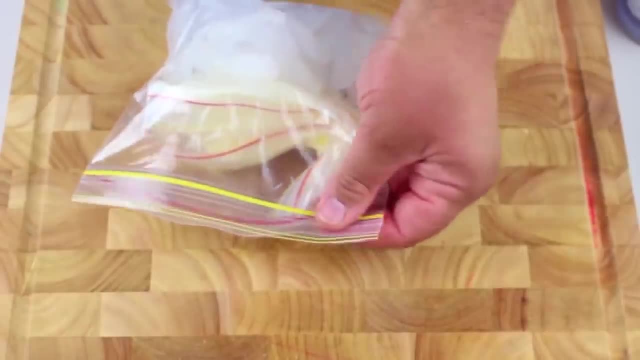 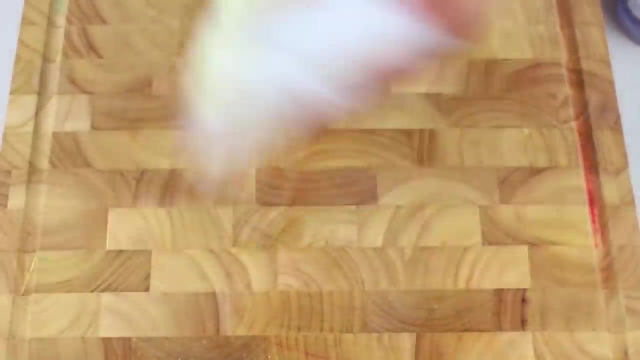 a larger bag. fill it with ice and salt, along with the smaller bag. Now shake vigorously for 7-10 minutes. This is where the kids come in. Eventually it'll come to a semi-soft consistency like ice cream. You can also make butter just by shaking heavy cream- No ice. 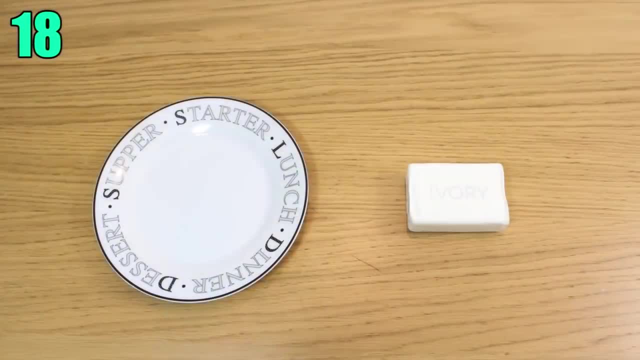 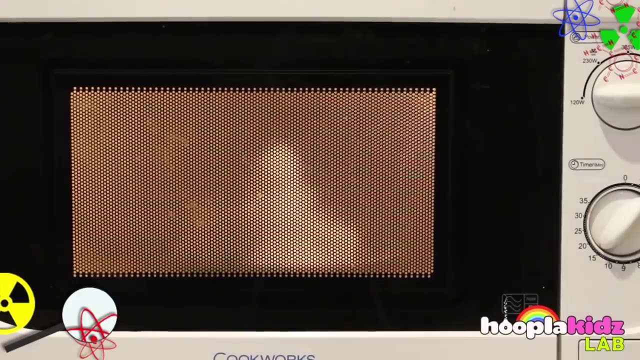 needed 18.. Puffy Soap: Ideally you want some sort of soap that can float in water. Ivory is most common. It's because just the brand of soap has air trapped within it, so obviously it expands. After you take it out of the microwave, however, let it cool just a little bit and you can. 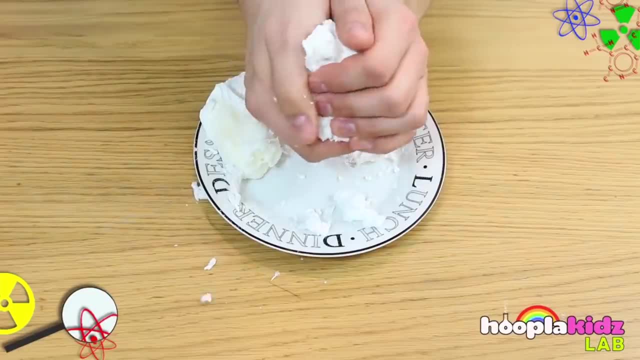 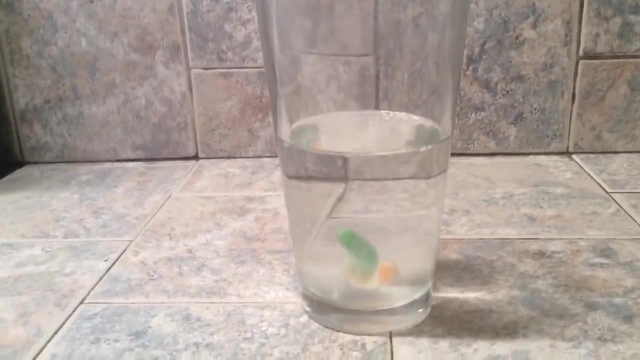 squeeze it back into regular soap. You don't want any air trapped in it, so just let it cool down. 17. Dancing Gummy Worms. Ok, this one is super easy. Simply cut a gummy worm into quarters and place them into a cup. 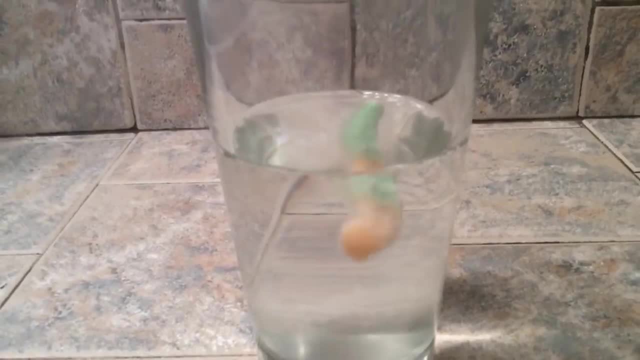 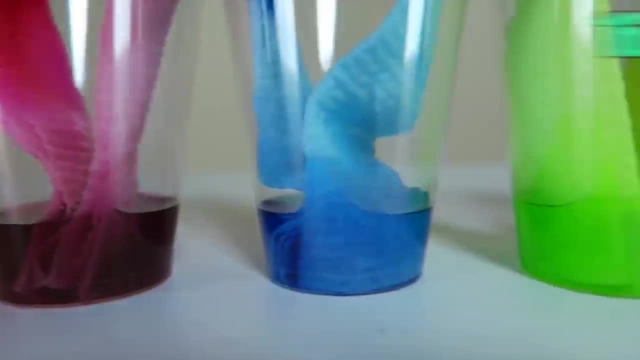 of salt water for around 15 or more minutes, Then drop them into a glass of vinegar and they'll start to spin and dance around. It's very weird to watch, but also very satisfying, so I would definitely recommend this one- 16.. Awesome Color Blending. 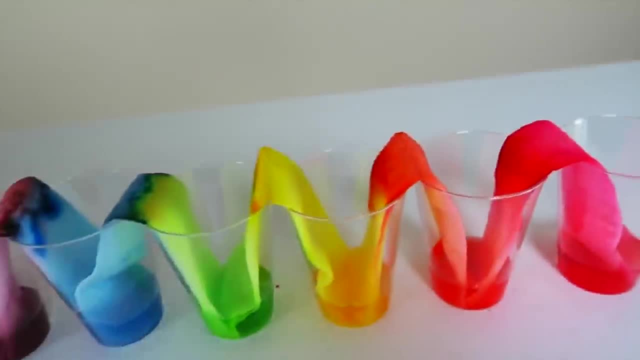 For this experiment you'll need 7 cups- preferably clear, red, yellow and blue food coloring and a paper towel. Fold the paper towel in half and then fold the paper towel in half. The paper towel can be folded in half long ways and fill every other cup with water and your 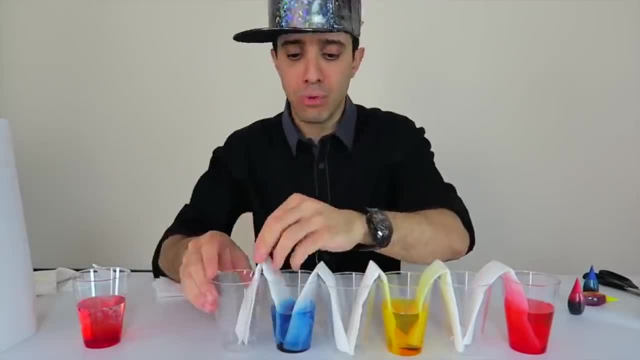 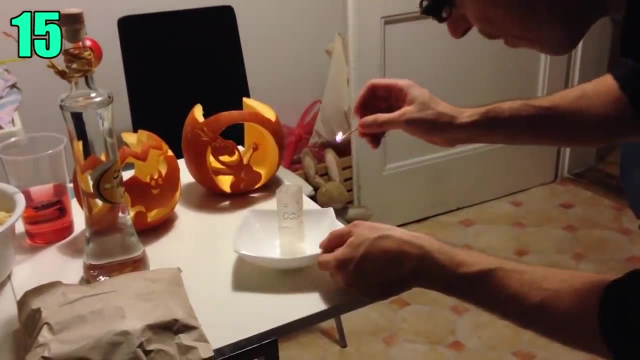 food coloring like so. Then fold each paper towel into opposing cups. Now watch the magic happen. 15. Teabag Ghosts. There's not much to it really, to be honest. Just cut off the top part of a teabag with. 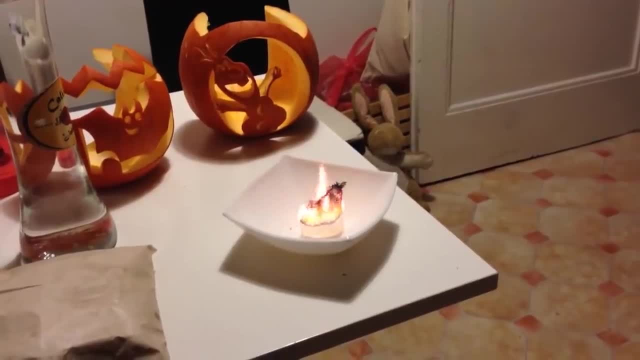 a staple and empty it out, Then balance it on a plate and light it on fire. It makes for a great Halloween trick if you put the effort in and draw a ghost on the teabag. 14. Sticky Ice. For this you'll want to use a paper towel. If you don't have one, you'll. 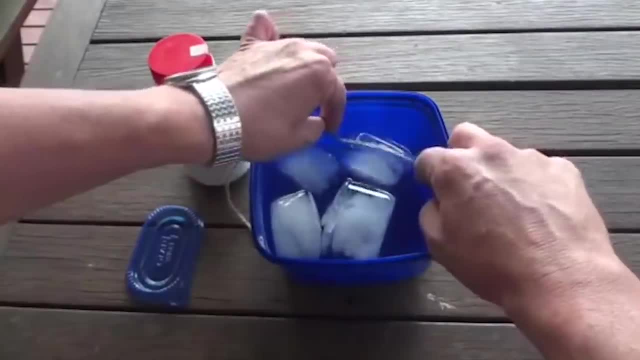 want to use a paper towel. If you don't have one, you'll want to use a paper towel. If you're doing this, you'll want to place some ice in a container with cold water, Lay some string over the ice, sprinkle some salt on it and leave it in the water for around a minute. 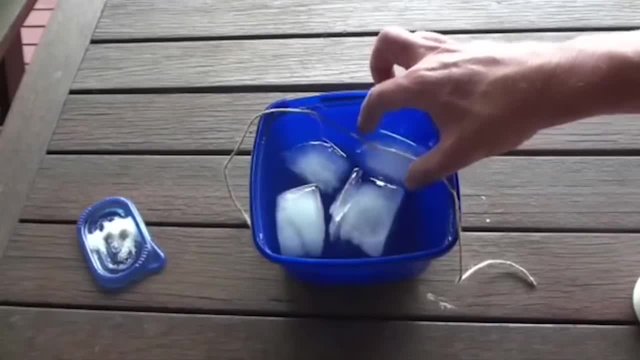 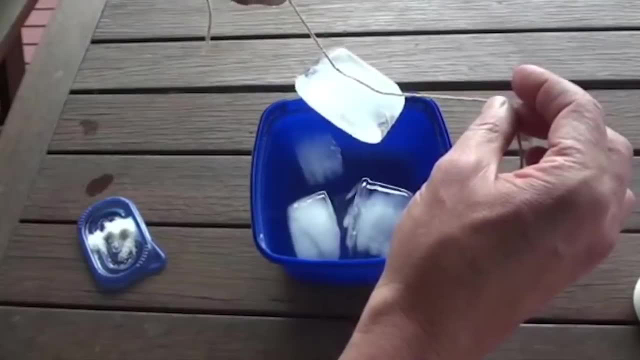 or two to allow the salt to wash away. The salt initially melts the ice, but once washed away, the water freezes around the string and attaches it to the ice cube. Lift up the string and the ice comes out of the water with it. 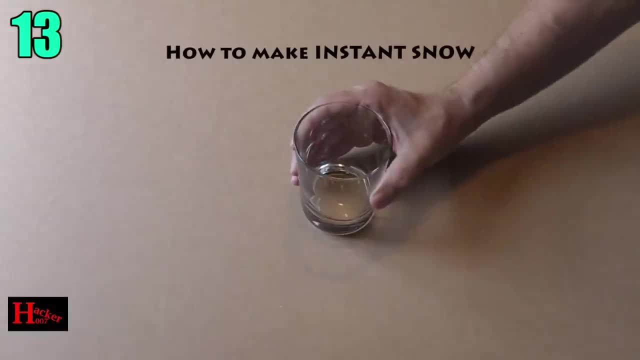 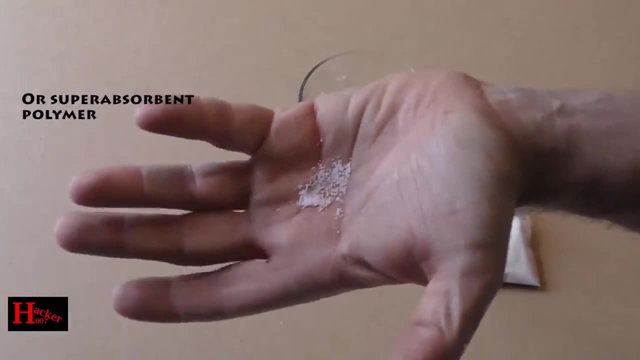 13. Homemade Snow. So for this one, all you need is water and sodium polyacrylate Sounds fancy, but it's easy to find online, Trust me. I actually tried to look it up and two links later I find it. 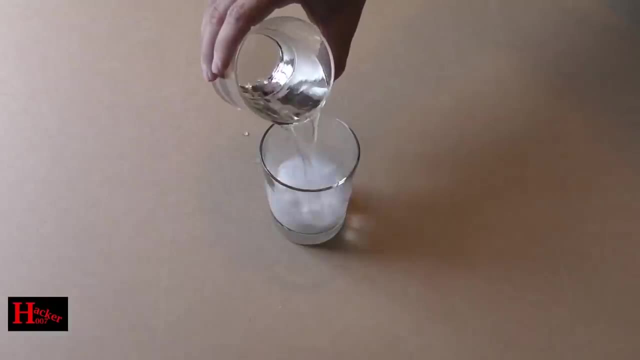 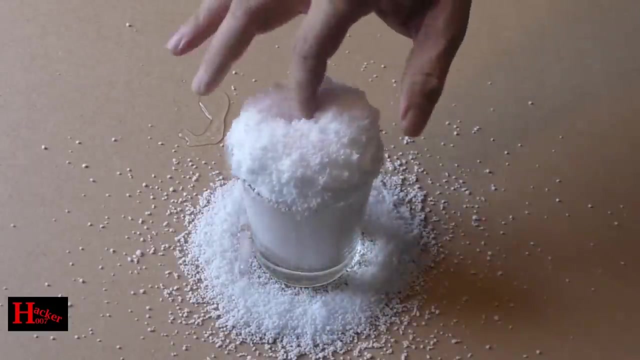 And what does this do? If you're looking for a good ice cube, this is the one you need. It absorbs water very quickly and in a large quantity, expanding the powder to make it look and somewhat feel like snow. So if you're ever looking to celebrate Christmas in July, 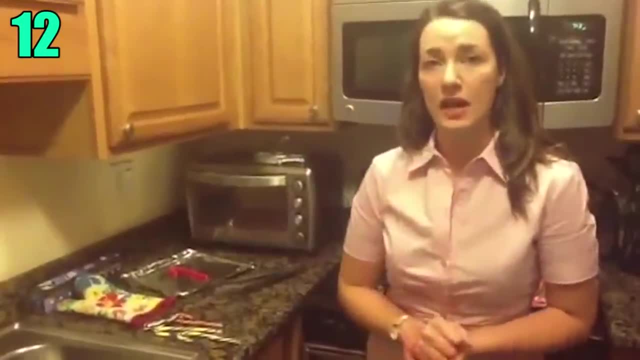 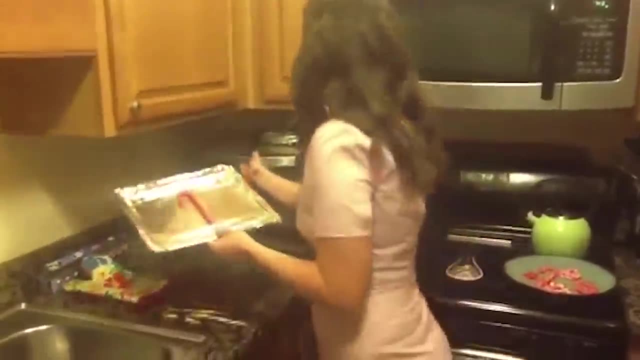 we've got you covered. 12. Candy Cane Molding. Tired of that classic. look, Here's how to make eating candy canes more interesting, if that's even a thing. Just place however many on a parchment paper covered baking sheet. Put them in a 250 degree. 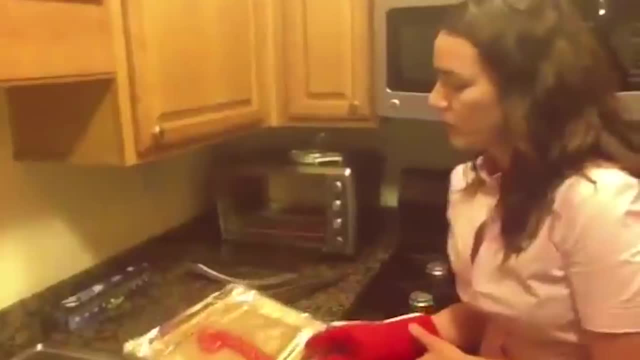 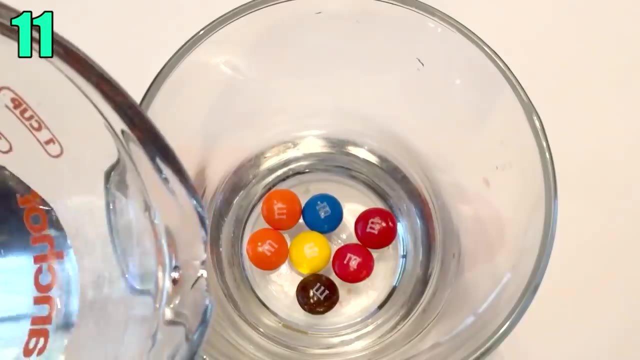 oven for 10 minutes. They'll be a little puffy but hold the shape wonderfully. This is great if you still have some leftover canes from the holidays, and Valentine's Day is fast approaching- 11. The Floating M- If you didn't know already, those M's on your M&M's are made up of edible. 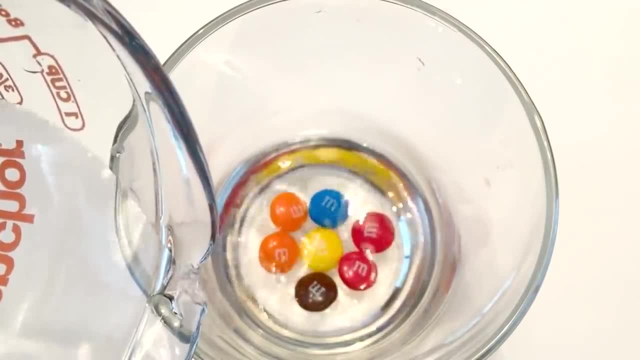 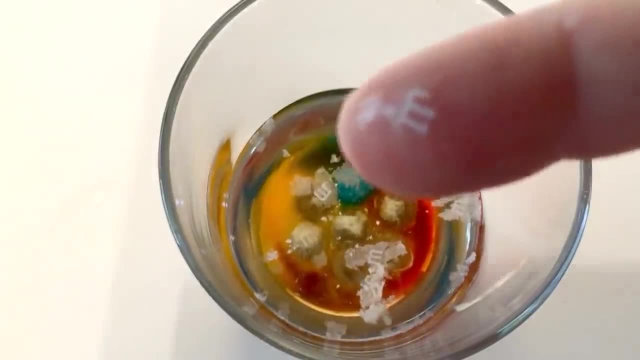 paper. So by placing a few M&M's in a glass of water, they'll eventually dissolve and after about 5-10 minutes the M's will begin floating and you can pick them up with your fingers. Somewhat of a useless science experiment, but it's really cool to do. I've done it. 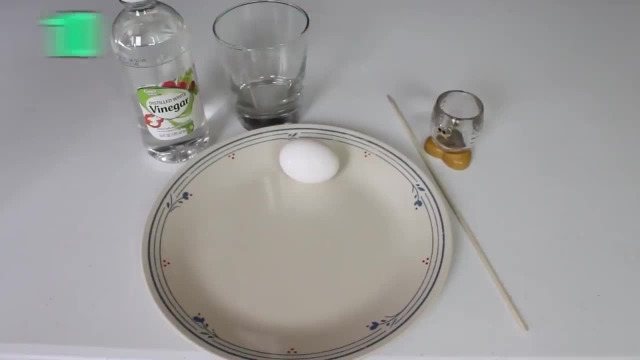 before and I absolutely recommend it for the younger ones. 10. Egg Eruption. So we've already mentioned in a previous video that egg eruptions are a very common phenomenon in the world. But if you don't know what egg eruptions are, 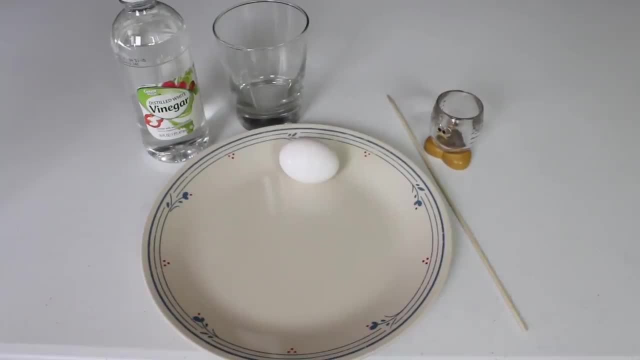 you're probably wrong If you don't know what egg eruptions are. you're probably wrong If you're not familiar with the science experiments. the list how you can make rubber-like bouncing eggs. But as it turns out, there's actually more to it. So after you've gotten your bouncy, 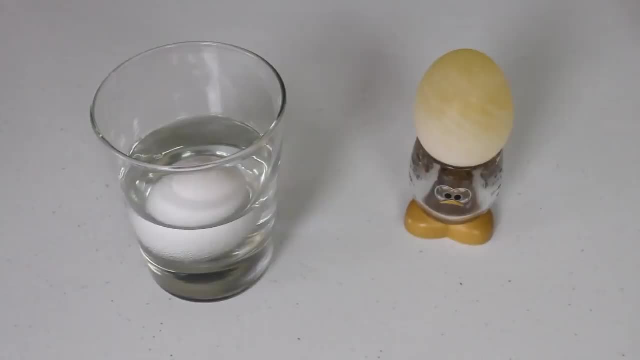 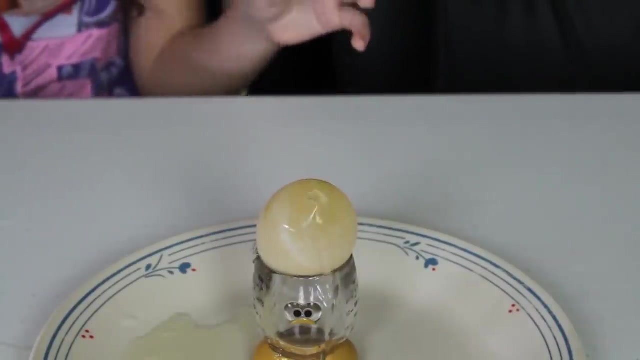 egg by laying a raw egg, sit in vinegar for roughly around 24 hours, rest it on an egg holder or something similar and poke a hole into it. Boom, you've got yourself a mini eruption. Super simple and messy, so sorry. parents might want to keep some paper towels. 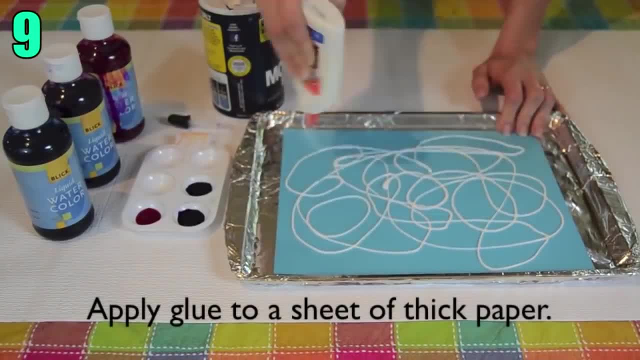 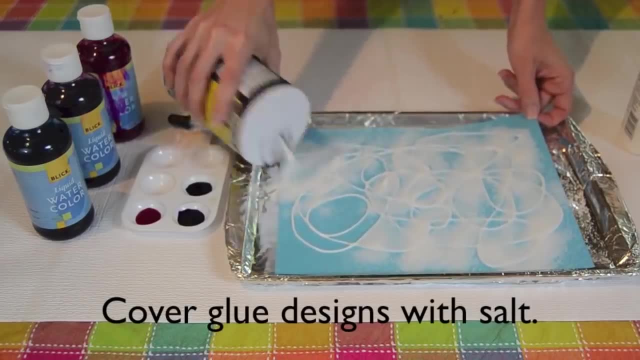 around 9.. Watercolors: This one is super cool, and if you're ever feeling extra creative, well, this is the one to do. What you'll need to start with is getting liquid white glue and use it as your pencil. Literally draw whatever you want with it over a canvas. Then, before it dries, sprinkle. 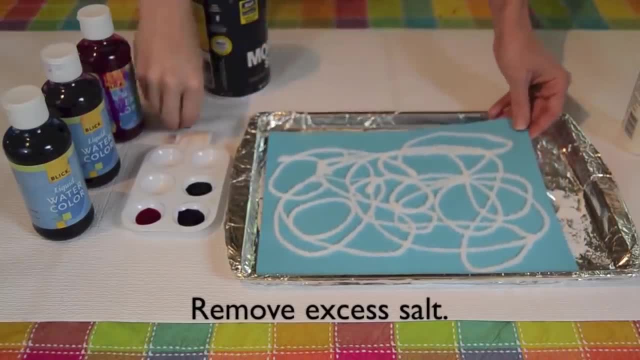 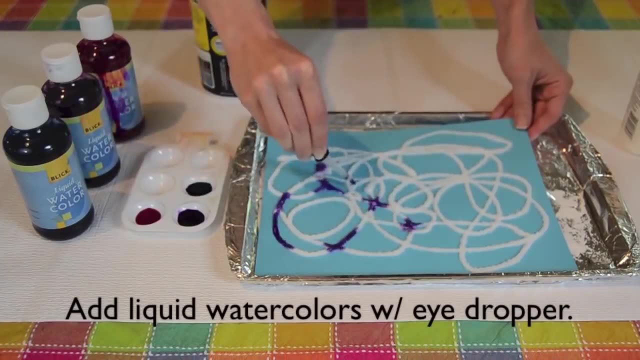 salt over it and remove any excess salt. Next, you'll need a source of watercoloring. So for something quick, just mix water and food dye and drip it over the salt where desired and it looks like crystal art. Pretty simple, but again, really awesome to try. 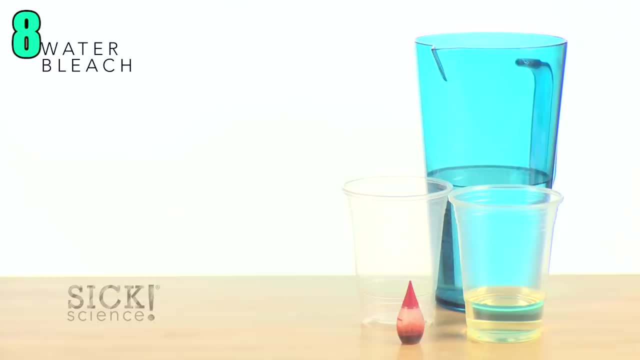 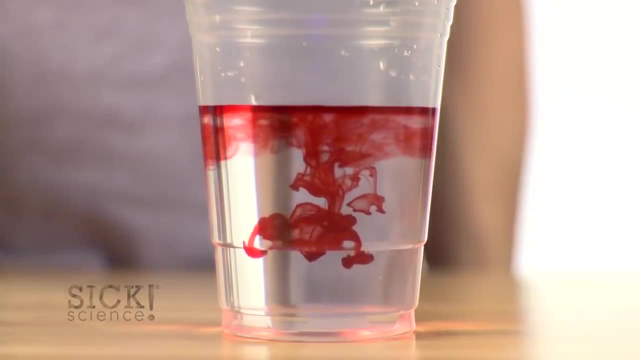 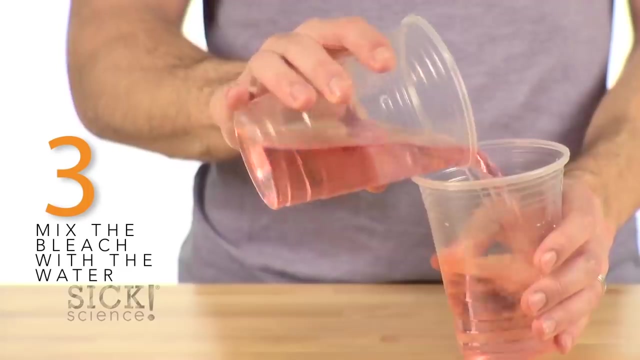 8. The power of bleach. If you've ever wanted to witness firsthand what bleach is capable of, here's your chance. Mix in some water with food coloring, in this case red. Then mix it with some bleach in another cup. Repeatedly switch the fluids back and forth from cup to cup to cup to get. 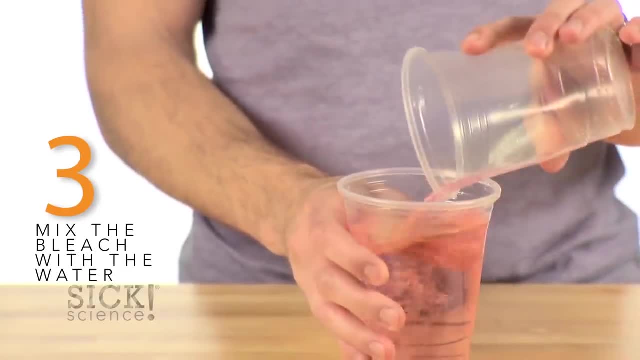 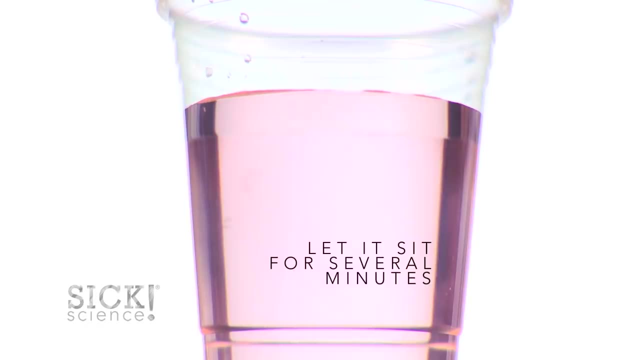 a good mix going and just let it sit. Over time the red will fade away, like in your stained clothing. This is because the bleach oxidizes the molecules from your food coloring to the point of transparency. Sounds confusing, but it's really cool to watch. Also, I probably 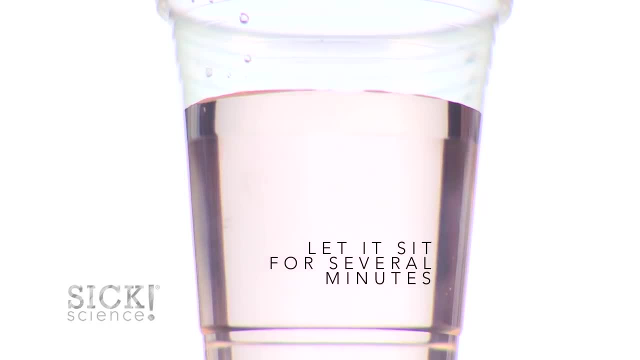 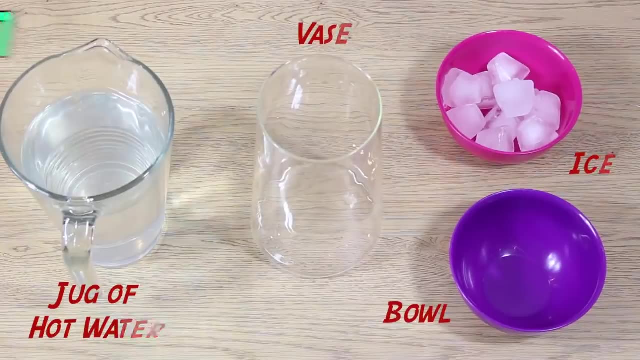 shouldn't have to mention this, but make sure your kids don't drink this, Or you, You're going to want to make sure you drink this. 7. Homemade rain. If you've ever wanted a close-up visualization of how rain forms in, 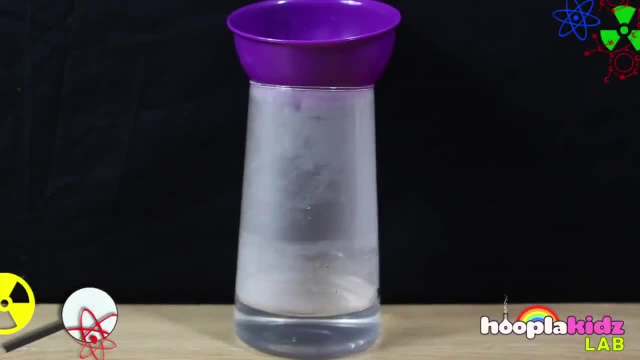 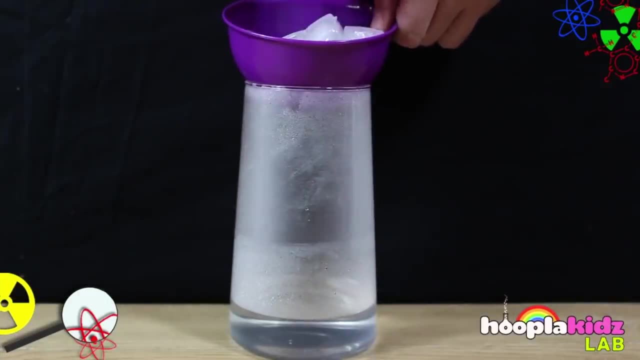 our atmosphere. here's an experiment just for that. Simply boil up some water into a vase and place a bowl over it until it becomes somewhat foggy. Then fill the bowl with ice. Soon enough, hot air within the vase will react with the coolness of the bottom of the. 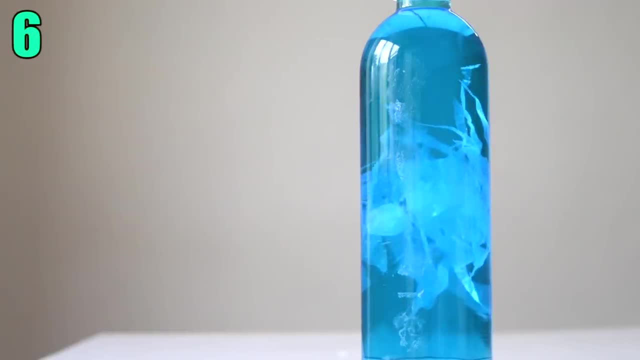 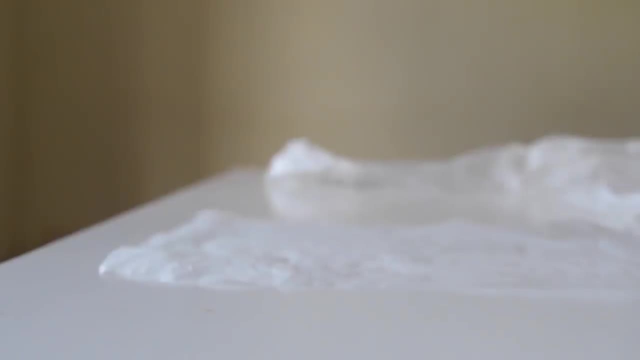 ice bowl, creating condensation. 6. Jellyfish in a bottle. Start this one off by mixing food coloring into a water bottle. Next, cut out a square from a piece of paper and place it in a glass container. This will be the jellyfish's head. Then cut apart the lower half to give it some stringers. Finally, 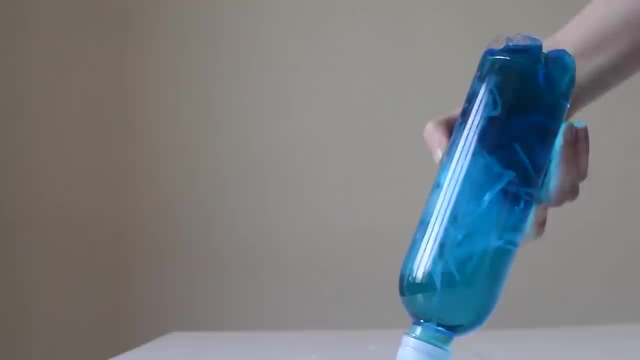 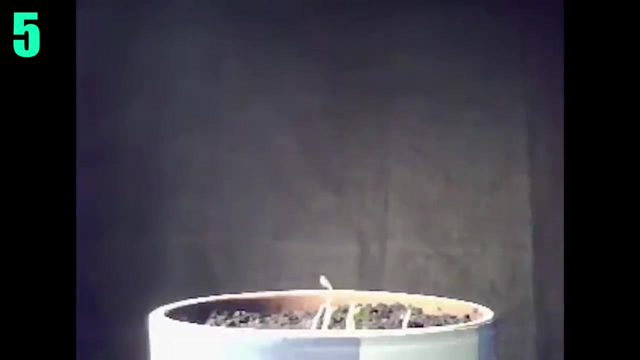 put our little jellyfish into a bottle and add some final bits of food coloring. Pretty cool, if you ask me, And there you go. 5. Plant growth manipulation, or in other words, tropism. It's a really cool experiment to see how a plant's growth is affected by where they receive sunlight, In this case, the plant's source of light was changed from side to side. This is a really cool experiment. This is a really cool experiment to see how a plant's growth is affected by where they receive sunlight. In this case, the plant's source of light was changed from side to side. 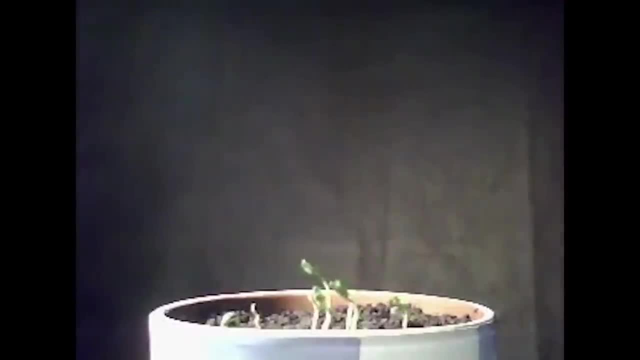 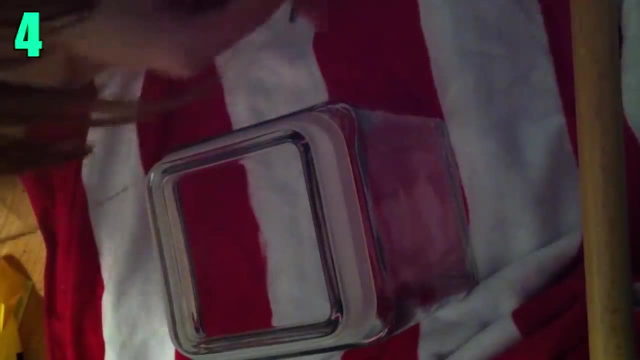 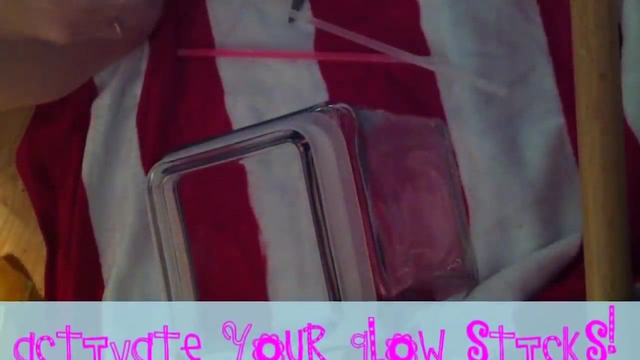 So every 10 or 15 minutes. itTom taverää 2 times in a day. 3. Firefly jars. Ok, this one is extremely simple and pretty much anyone can do it. All you need is a clear jar and glow sticks. Cut off the edges of your glow stick and shake them. 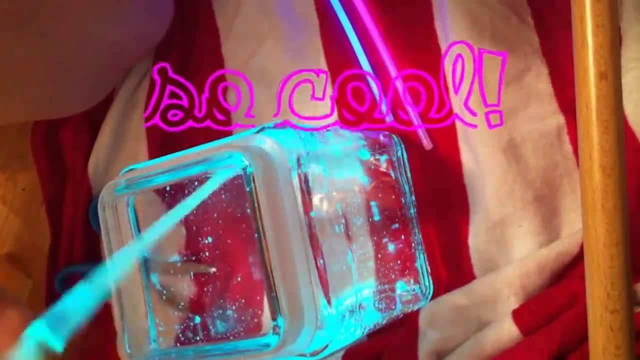 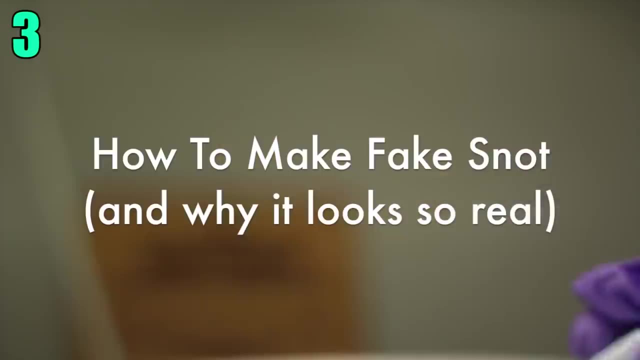 like crazy into the jar. so they go all over And it's pretty cool looking and neat for parties. Form added effect: dust some glitter into the jar as well. That makes it look crazy. 3. Snus, It's not. 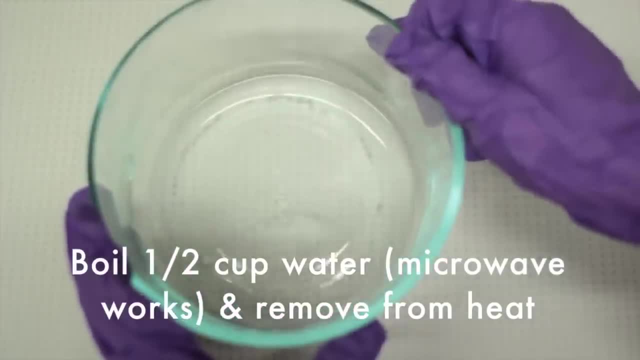 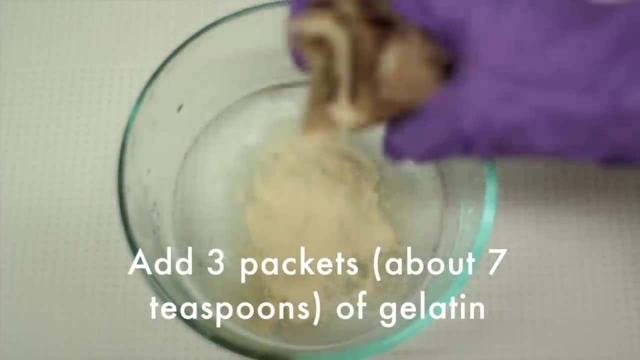 I was going to make a joke, but it's not really that funny. Ha ha ha ha, I'm dead inside. Anyways, this is basically our regular take on making slime, but with the added benefit of giving it its snotty texture. 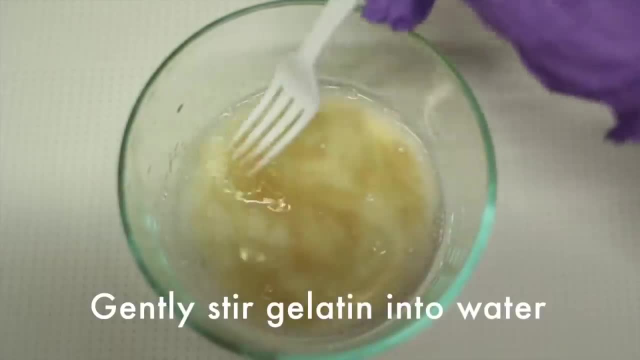 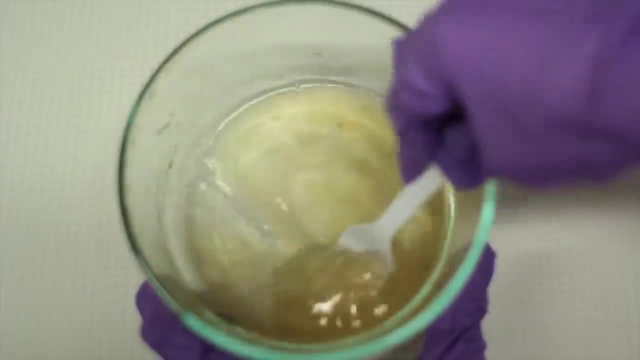 Just add seven spoons of gelatin to a half cup of hot water and stir very gently. Then add a quarter cup of corn syrup and stir until you're happy with the consistency. Add green food coloring. if you want more of a snotty cartoonish, look to it, but be warned. 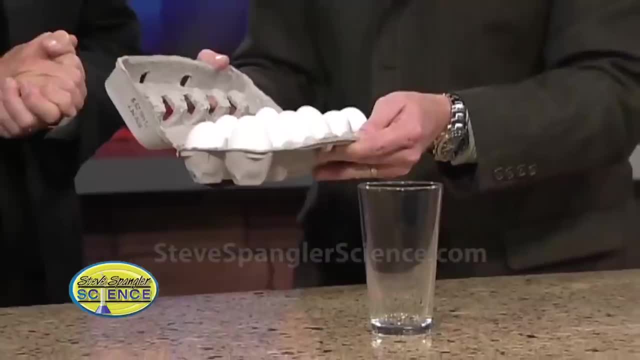 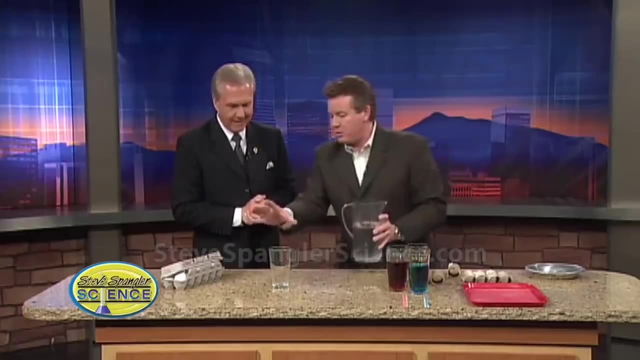 this gets pretty gross looking. so if you're queasy, just watch out. Number two: Inertia. Basically it means if you don't apply a force to an object at rest or in motion, it will stay at rest or at that same motion along a straight path.